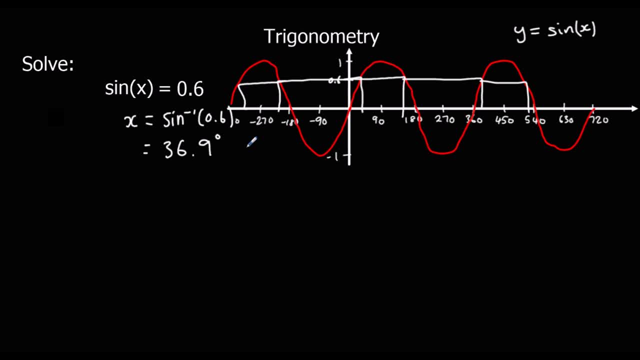 So we've got one answer from the calculator and we need to be able to get to generate more answers. So what we use is well we use a knowledge of the graph. So we only need to look at the first 360 degrees because this wave repeats every 360 degrees. So we get the same wave 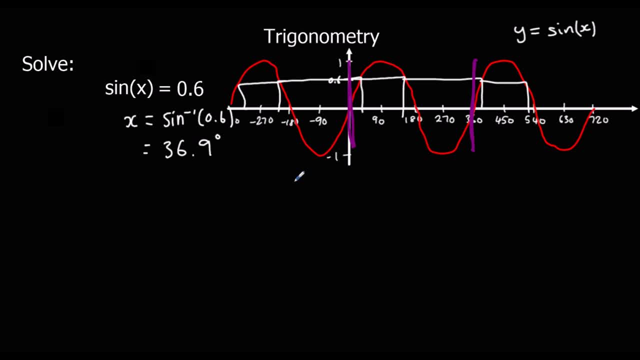 every 360 degrees. So if we find the two answers, we get the same wave every 360 degrees. So we need to be able to get the two answers, we've got one answer. So thisıy can NI3bEn we could just add 360 onto them or take 360 off of them to generate more answers. So that's the first answer we've got here, what's the second answer? 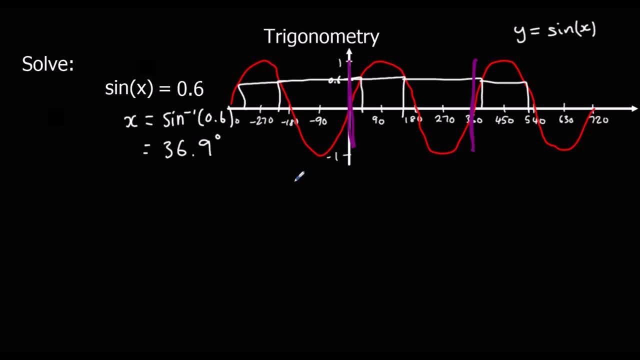 So we use symmetry. So this distance here because of symmetry is the same as this distance here. 36.9 is our first answer. so here we've got a 번째 here. That'sился DPp2Y. 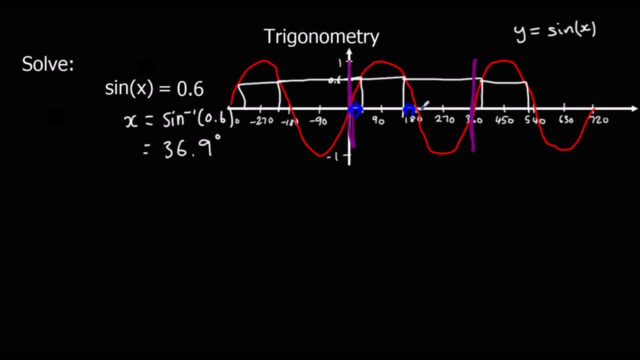 So what is that step here? It's just the last answer of the graph. So thetatanson things we can calculate like that simultaneously bilust chemistry anyways relative degrees of variance average times. So there are three other values here and along that line it's like I couldn't use it any longer let's just do that from this graph. So this is our input reflex.utm and so we give that to theivi here applying our eigen preach on clockwise 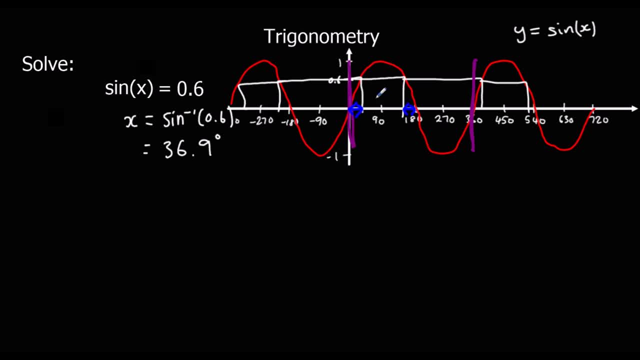 here? 36.9 is our first answer. That's the distance here. So this distance is 180 minus the first answer. So 180 minus 36.9, which is 143.1 degrees. So the first answer is 36.9. Our second answer is 143.1. And then if I wanted to find this next answer here, so if I wanted to find this one here, that would be 36.9 plus 360. So we'll have 396.9. 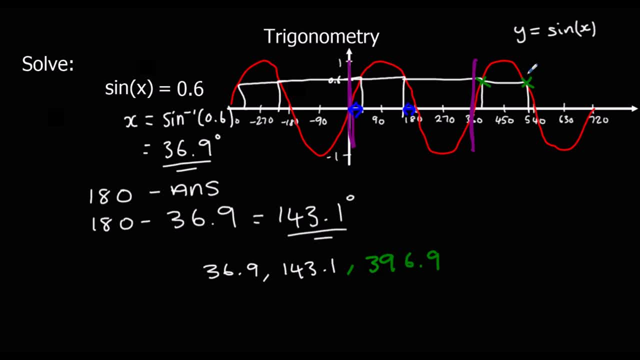 And if I wanted the next one, that would be 143.1 plus 360. So we'll have 396.9. So 503.1. And I could do the same thing going backwards. So if I wanted this one here, that will be 143.1 minus 360. And the one before that would be 36.9 minus 360. So I could keep adding on 360 or taking off 360 from both of the two, the first two answers from both of those. And I can generate every answer for sine x equals 0.6. 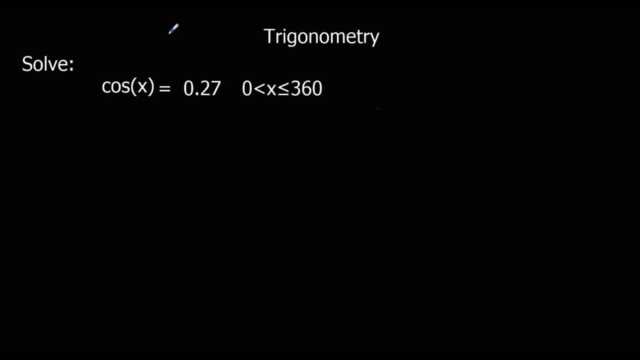 Okay, so let's look at a cos question now. So the first step is going to be the same. We're going to type into the calculator, shift cos, 0.27. And that will give us the first answer. So shift cos 0.27 gives us 74.3. 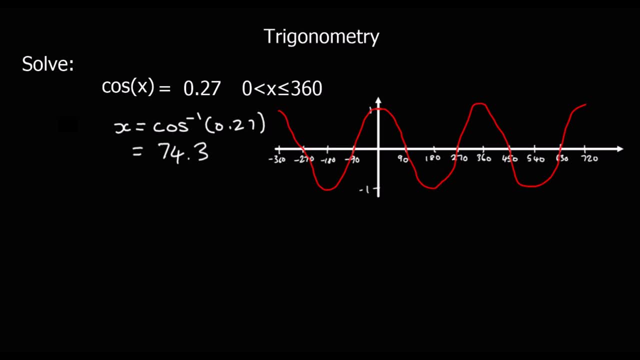 So that's the first answer. So we look at the cos graph now. Now again, cos is the same as sine in that it repeats every 360 degrees. So we're just going to look at the first 360 degrees. And we've got 0.27. So we've got it there and there. And we're again going to use symmetry. And we're going to say that this distance here is the same as this distance here. Our answer, our first answer there is that distance there. So the second answer for a cos question is 360. 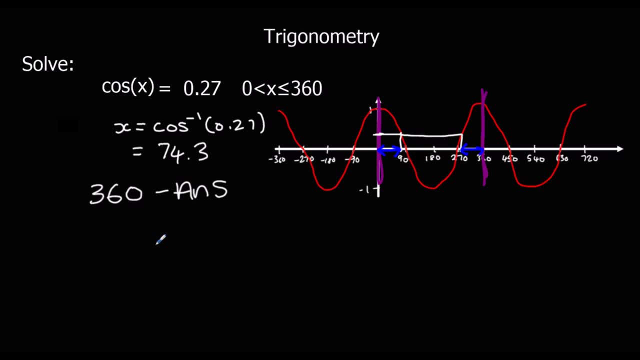 Minus the answer. So 360 minus our first answer, 360 minus 74.3 gives us 285.7. So there are our first two answers. 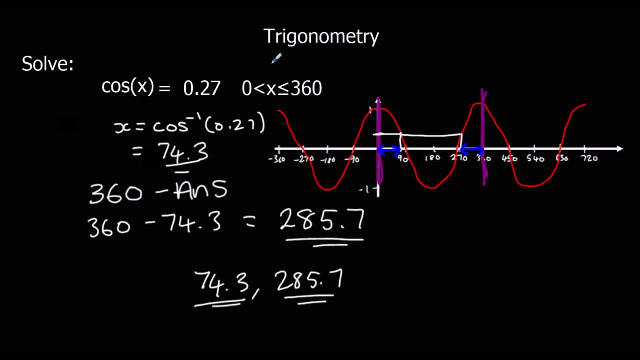 If I wanted to generate more, which I'm not going to because the question specifically said between 0 and 360. 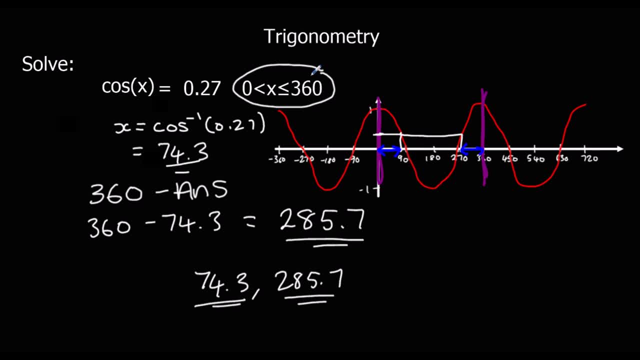 So there's only those two answers between 0 and 360. If I wanted to generate more, I'll just add 360 onto both of them or minus 360 from both of them. And I'll get more answers. 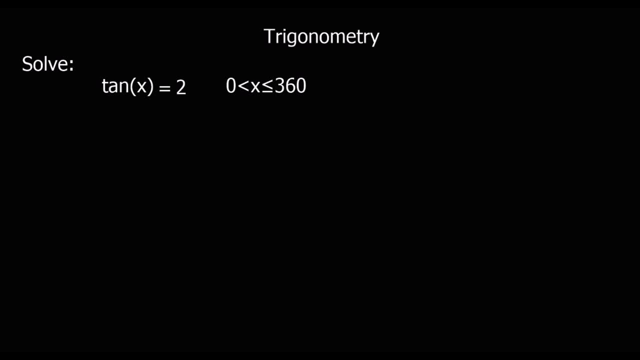 Okay, let's look at a tan question now. So again, the first step is the same. So shift tan 2. That will give us a first answer. For X, which is 63.4. So we've got our first answer of 63.4. And then we can look at the graph of tan. And the graph of tan is a bit different, but it's actually easier because the graph of tan repeats every 180 degrees. 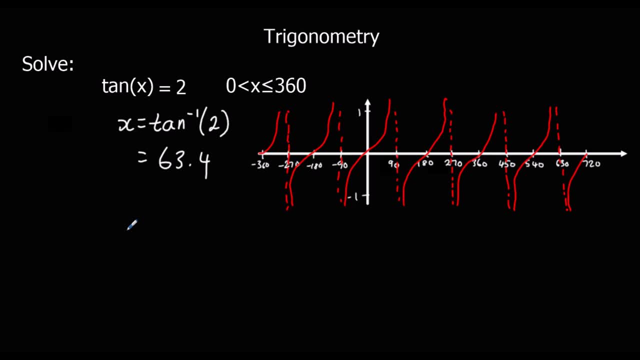 So all I've got to do is add 180 on. 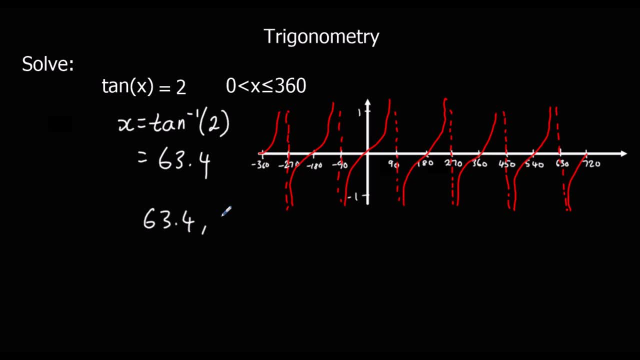 So. So 63.4 is the first one, adding 180 on, 243.4. 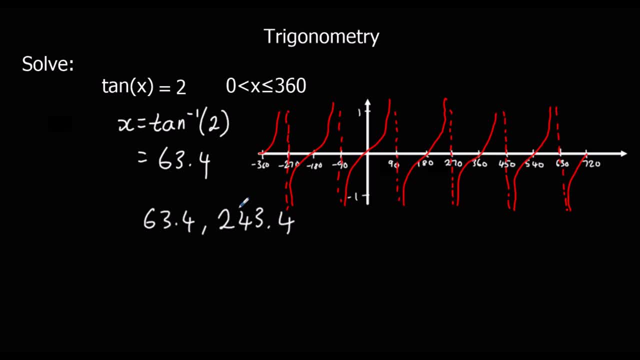 And I could keep adding 180 on or taking 180 off to generate more answers. 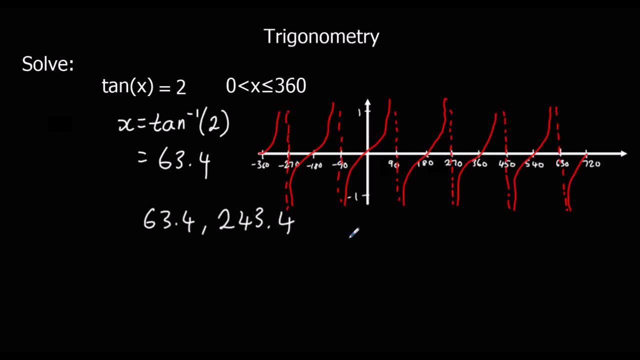 So with tan, we just have to add 180 and we can keep adding 180 or minusing 180 to generate the infinite number of answers. 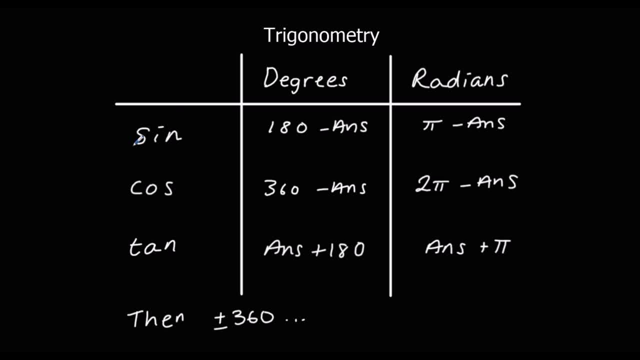 Okay, so let's summarise what we've just done. So for sine, after you get the first answer, you do 180 minus that answer. Or in radians, that's pi minus the first answer. For cos, it's 360 minus the first answer. 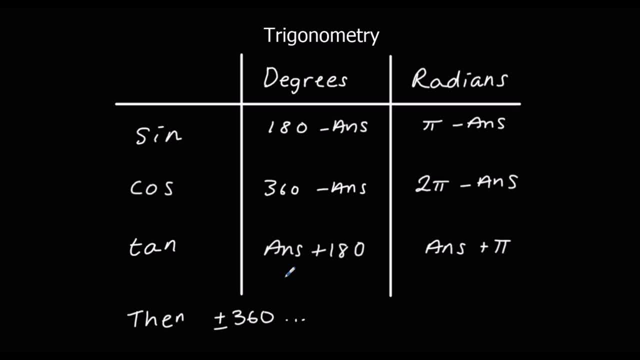 And for tan, we just keep on adding 180. Or in radians, adding on pi. Or taking away pi. And that will give us our answers. 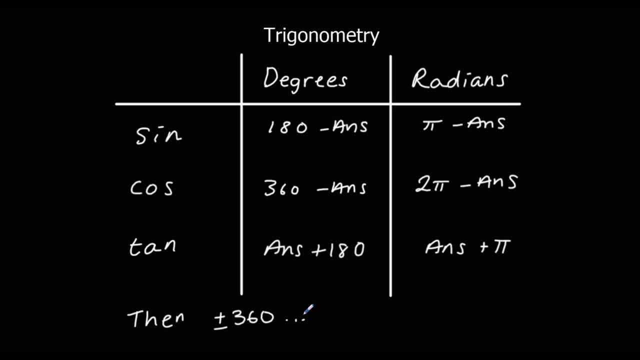 And then we can always add or take away 360 to generate more. 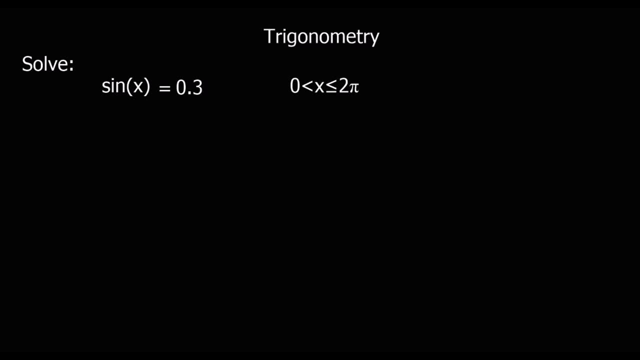 Okay, so let's have a look at a question. So here we've got solve sine x equals 0.3 for when x is between 0 and 2pi. So what that tells us, what this tells us, is we're going to be working in radians. So the first thing we need to do is make sure our calculator is in the radians mode. So it's got r at the top of the screen. 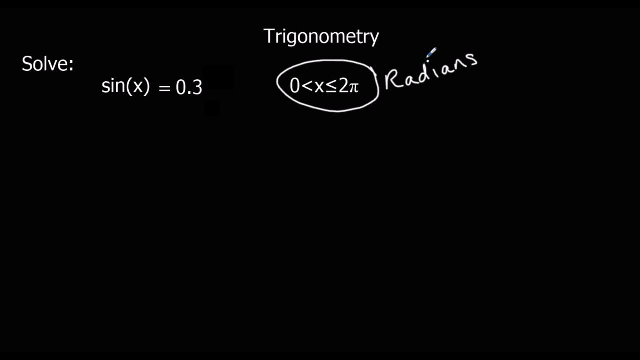 So we change our calculator into radians. And then we carry on as normal. 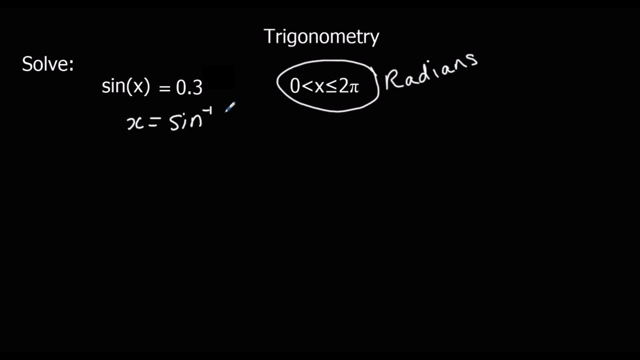 So x is shift sine 0.3. 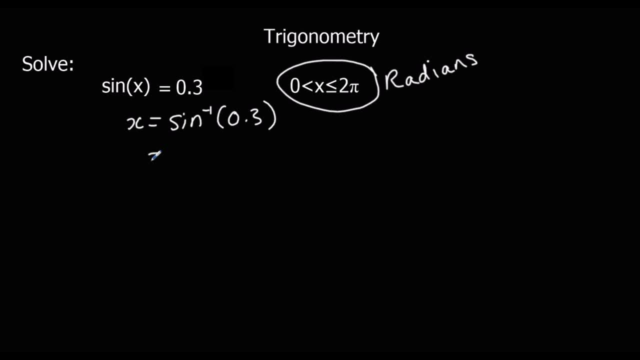 So shift sine 0.3. And that gives us 0.30. 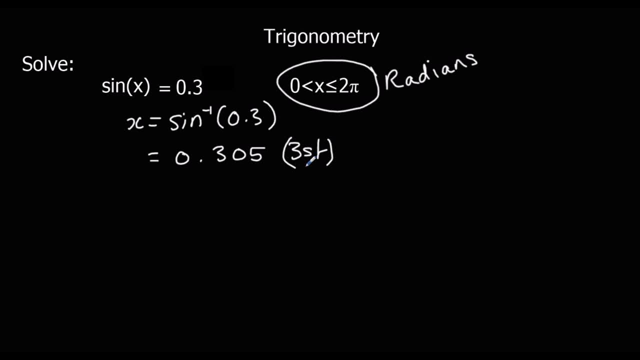 So that's our first answer. To get the next answer, in sine, that's 180 minus the first answer. So in radians, pi minus the first answer. So pi minus answer. 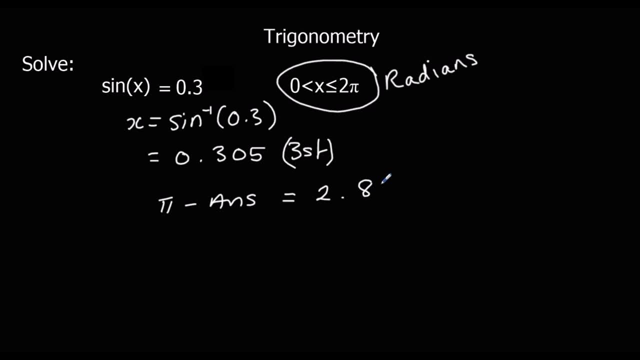 And that gives us 2.84 to 3 significant figures. 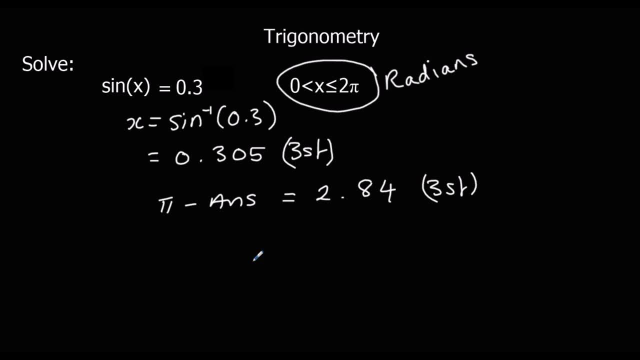 So between 0 and 2pi. That's both of our answers. 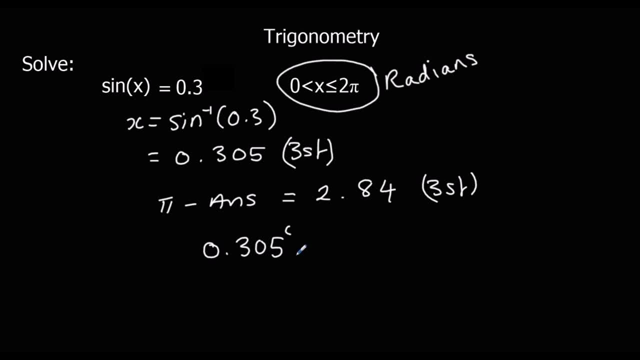 So we've got 0.305 and 2.84. 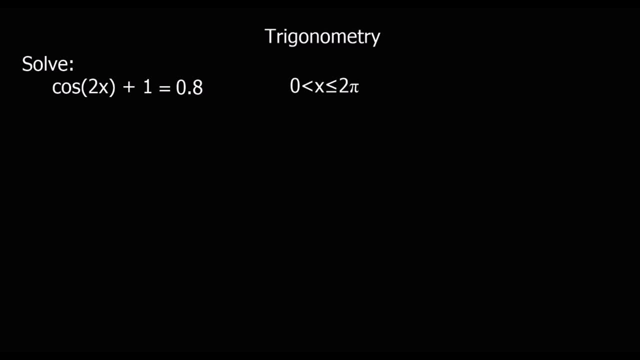 Okay, here we've got a question. Solve cos 2x plus 1 equals 0.8 for between 0 and 2pi. So it's between 0 and 2pi. So we know it's in radians. 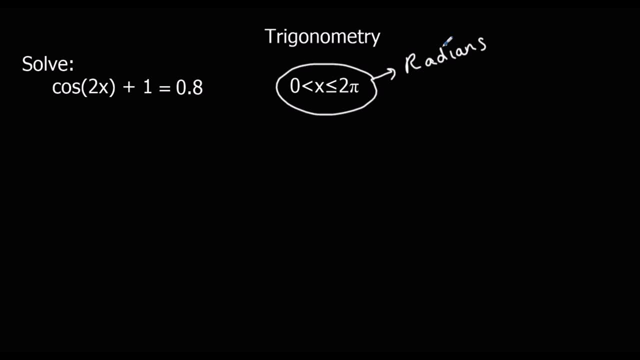 So we need to make sure that our calculator is in the radians mode. And then we can carry on with the question. 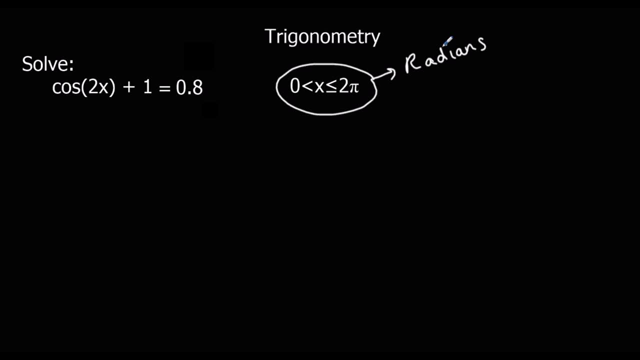 So cos 2x plus 1 equals 0.8. So we can't shift cos. We can't do the inverse of cos. Because there's also a plus 1 on that side of the equation. So we're going to get rid of that first. And we're going to do that by subtracting 1 from both sides. So cos 2x equals. Minus 0.2. 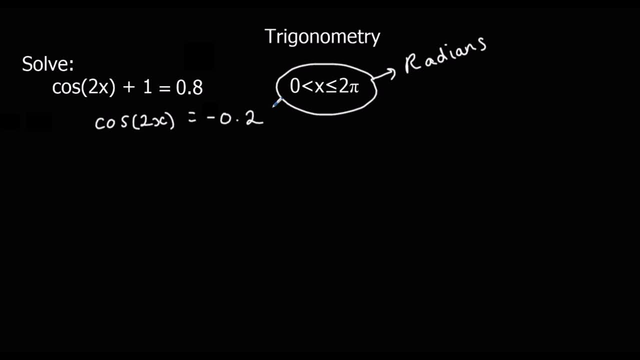 Now we've just got cos for the angle. So we can shift cos. Minus 0.2. 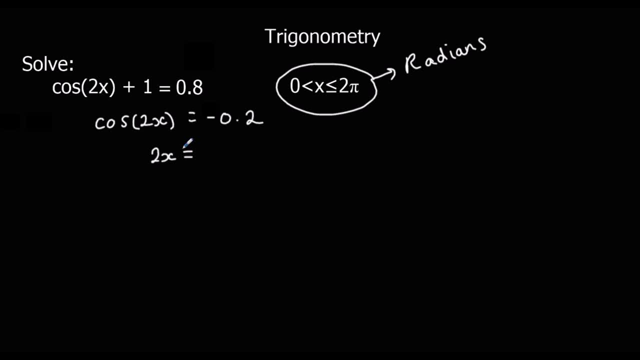 And we get our first answer. So 2x equals. We're going to write down the whole answer. Because we're not done using it in the question yet. 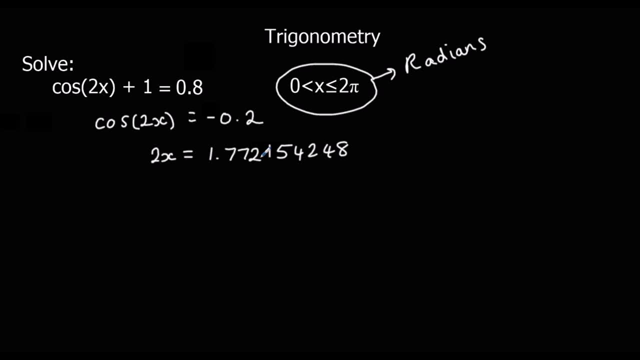 So 2x equals the first answer of 1.77215. 1.77215. 4248. Now we're in cos. To generate the second answer. 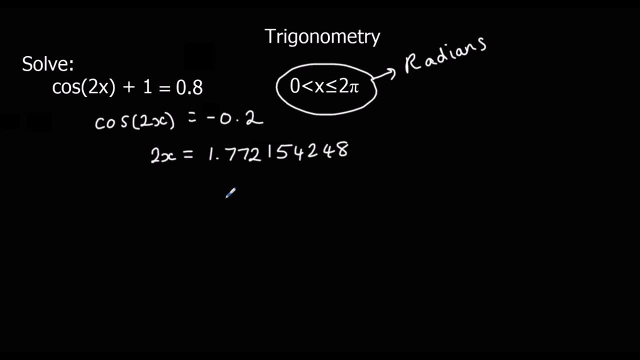 We're going to do 2pi minus the first answer. So 2pi minus the first answer. 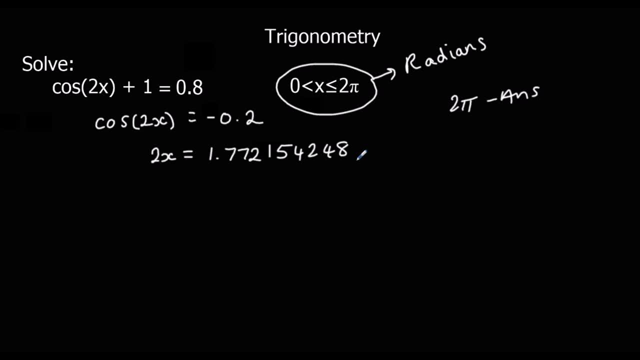 2pi minus answer. And that gives us 4.51103106. So we've got two answers now. 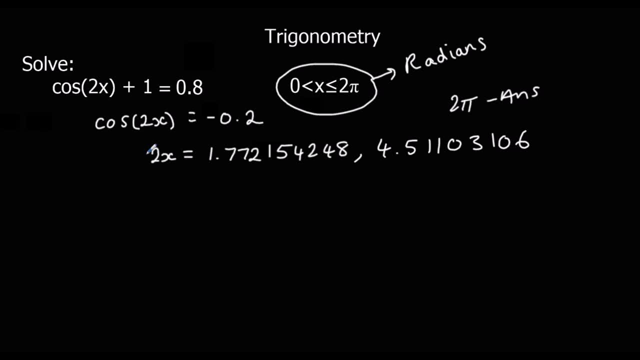 Between 0 and 2pi. But because they're 2x. We're going to have to half them. 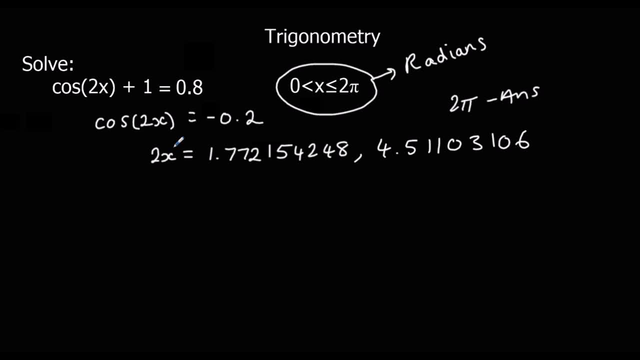 So we're actually going to need to generate more answers. So that when we half them. They're between 0 and 2pi. 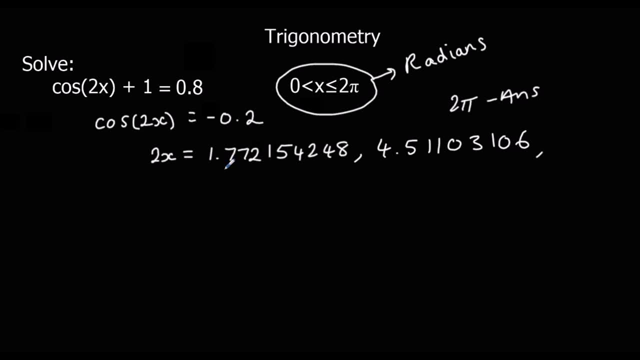 So we're going to get a third answer. So we're going to take the first one. And add 2pi onto it. 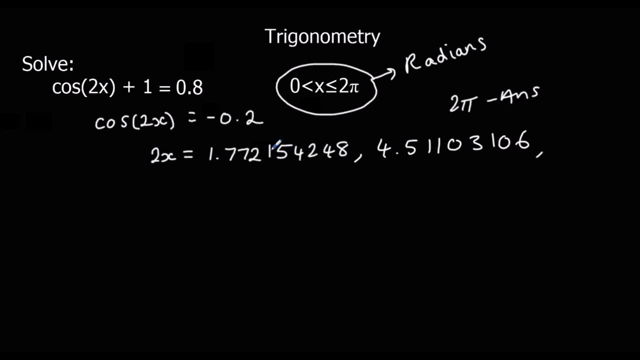 So take the first answer. Add 2pi. And you should get 8.0. 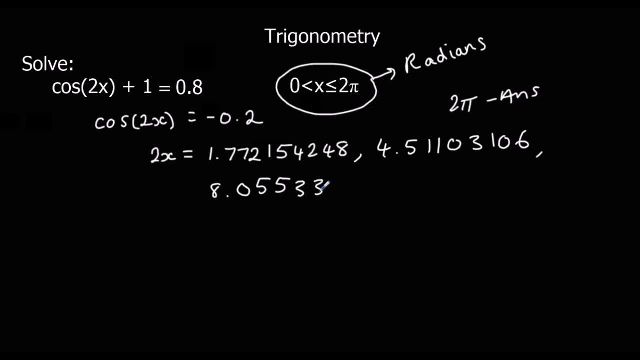 So that's going to give us. 10.3355. 3.39555. 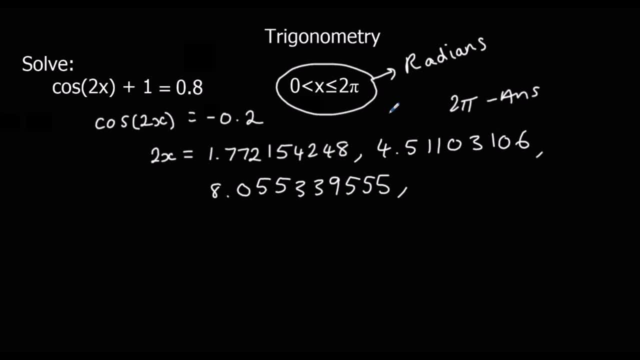 And we're going to take the second answer. And we're going to add 2pi onto that as well. So that gives us. 10.79421637. 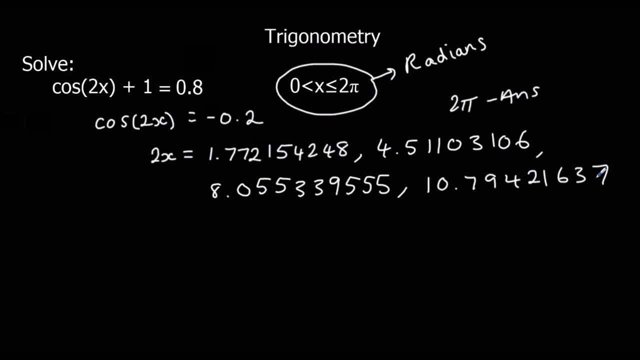 So now I've got my four answers. And I'm going to have to half all of them. To give me. My answers in between. Or my answers for x. So these are 2x. So I'm going to half them. And that will be x. 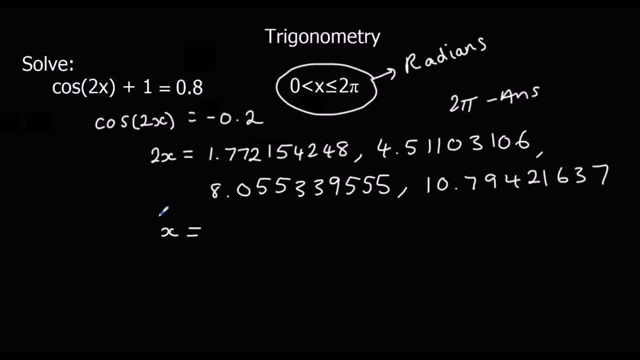 So. Halfing them all. So I'm going to give the answers to three significant figures now. 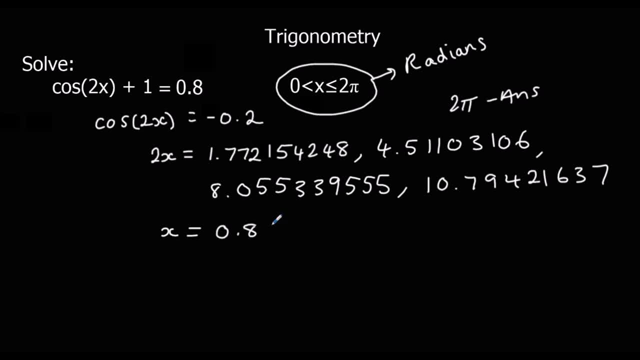 So half of the first one. 0.886. 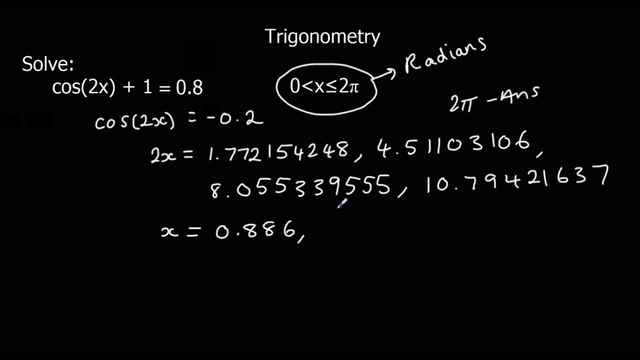 Half of the second one. 2.26. Half of the second one. 2.26. 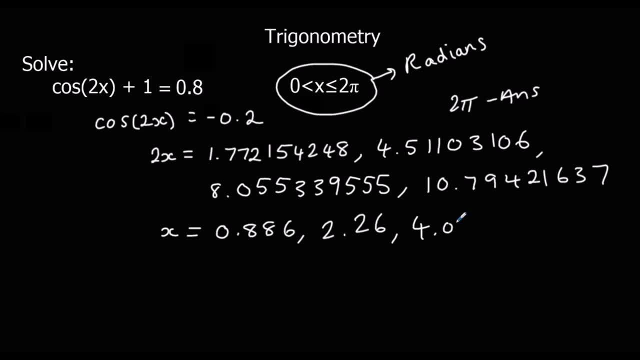 Half of the third one. 4.03. And finally. Half of the last one. Is 5.40. 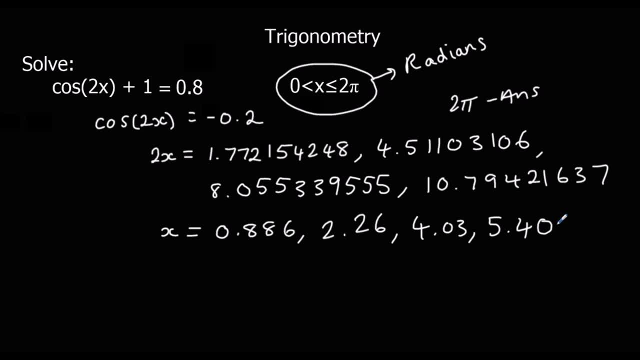 And there we have it. So four answers. In between 0 and 2pi. Okay so here's another question. 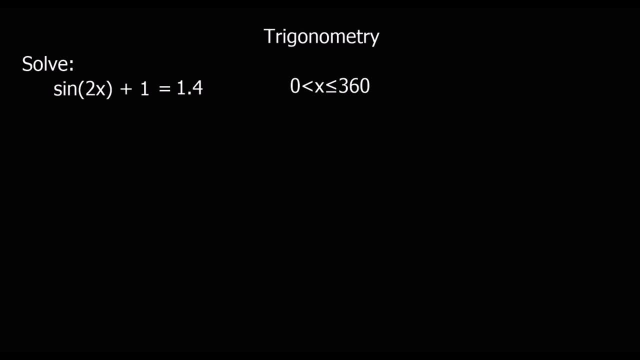 I'm going to pause the video. See if you can give this one a go. 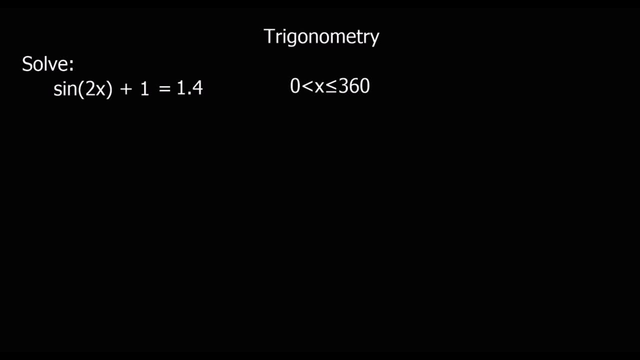 Okay. So the first thing. We need to notice. We've got sin2x. Plus 1 equals 1.4. Between 0 and 360. Degrees. So we're going to be in degrees this time. 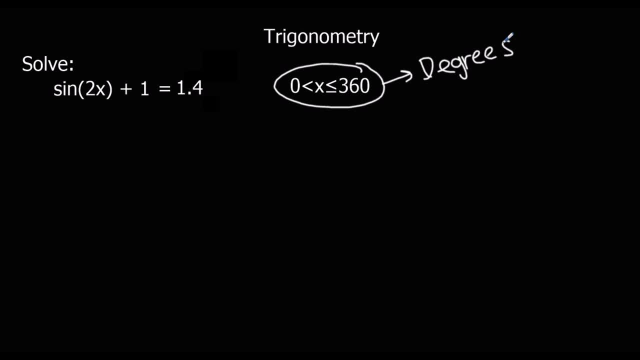 So. We need to change our calculator mode. 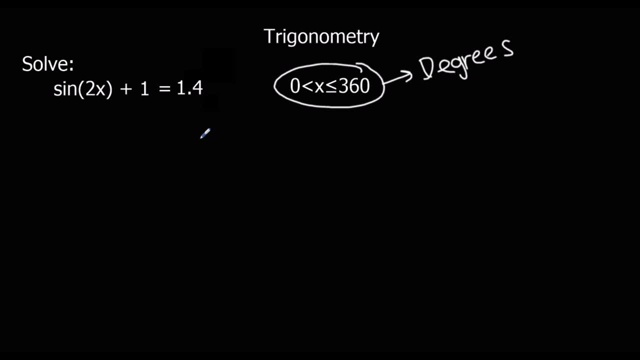 Back to degrees. So we've got. 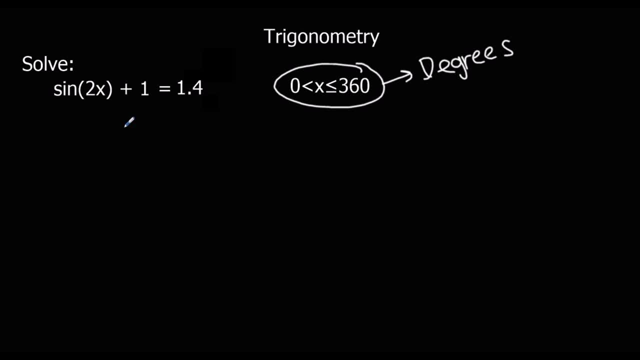 Sin2x. Plus 1 equals 1.4. So you want sin. With the angle. 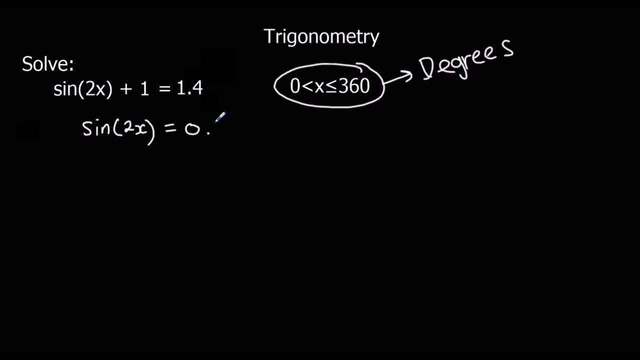 Of. So we're going to subtract 1 from both sides. And that will leave us with. Sin2x equals 0.4. 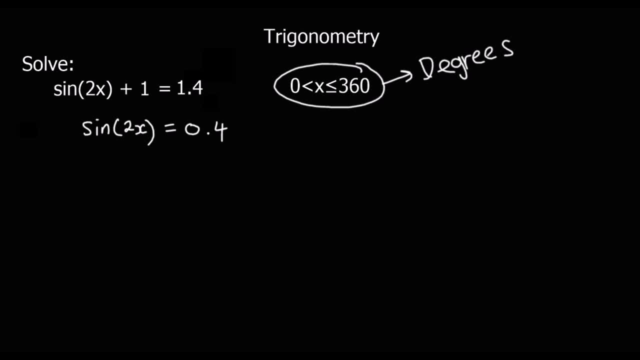 Then we can shift sign. So shift sign. 0.4. 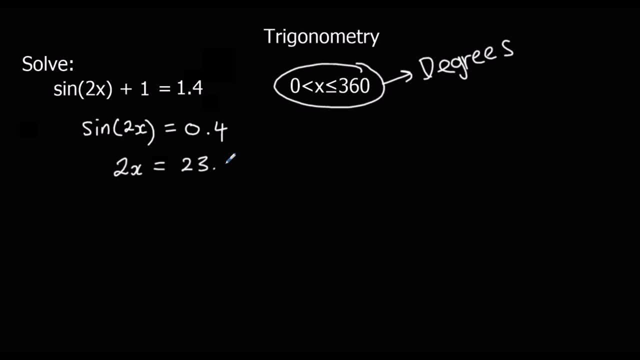 And. I'll write down the whole answer. 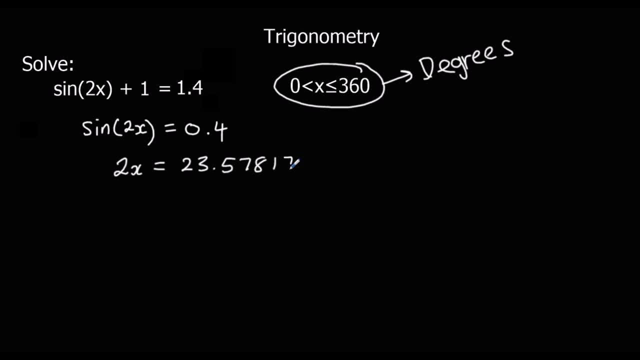 So 23. 578. 178. 48. So there's our first answer. Again. 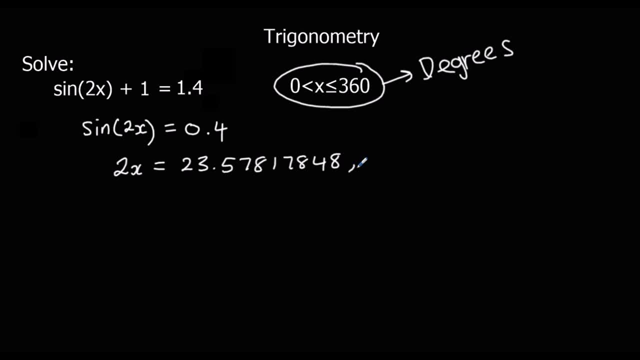 So we're going to do. 180 minus that. Which will be our second answer. Of. 156. 421. 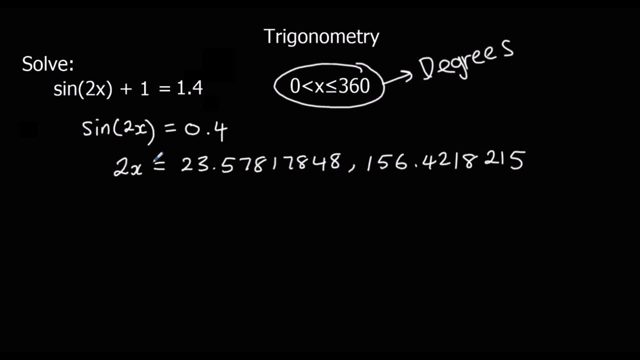 So again. It's 2x. 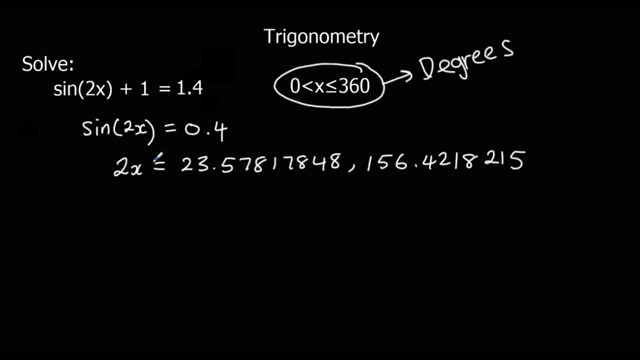 So we're going to have to generate twice as many answers. So. We're going to add 360. Onto both of these. 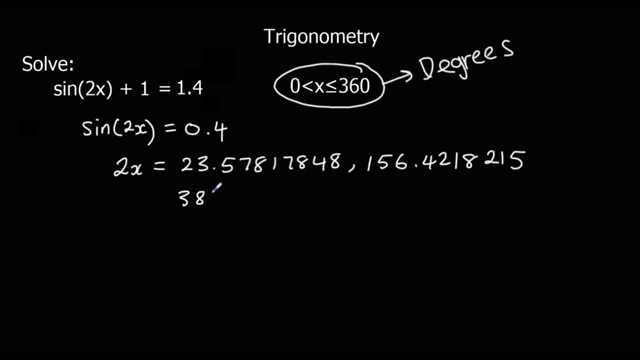 So the first one. Plus 360. 383. 57817. 848. And. 360. Onto the second one. 516. 421. 821. 5. 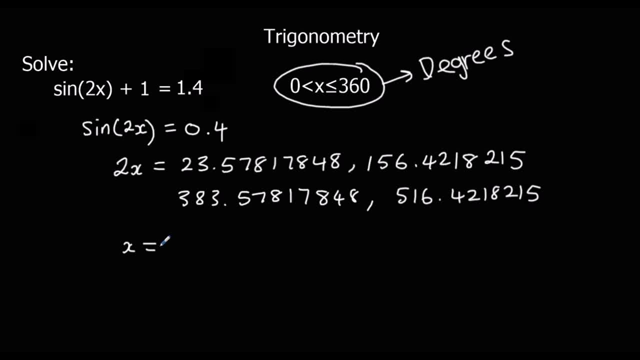 So that's 2x. So to get. Our answers. We're going to. Half them all.